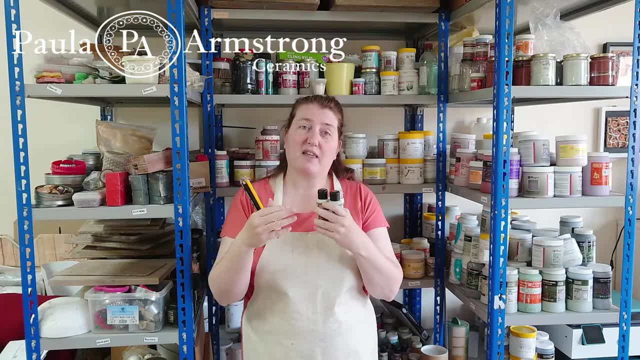 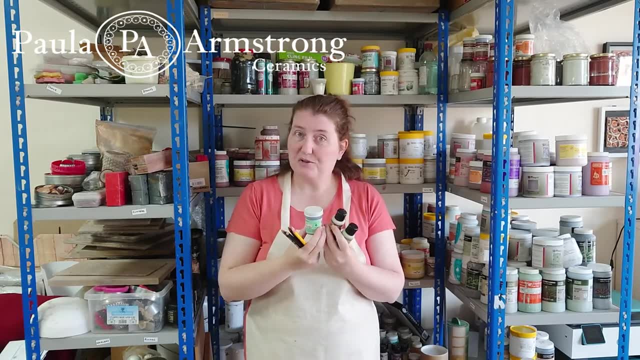 painterly. If you want something that doesn't have that brush stroke, that painterly effect, then you need more than one coat. There are other things you can do with them. You can do some inlay and you can do other sorts of 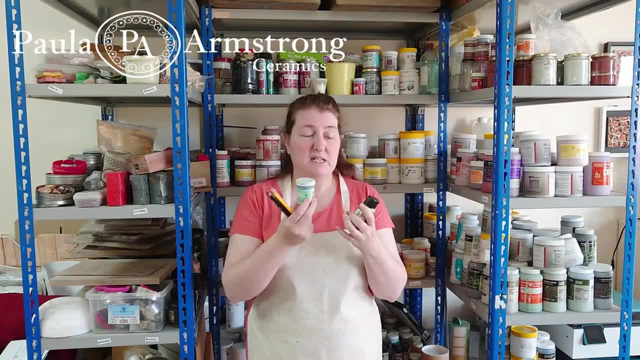 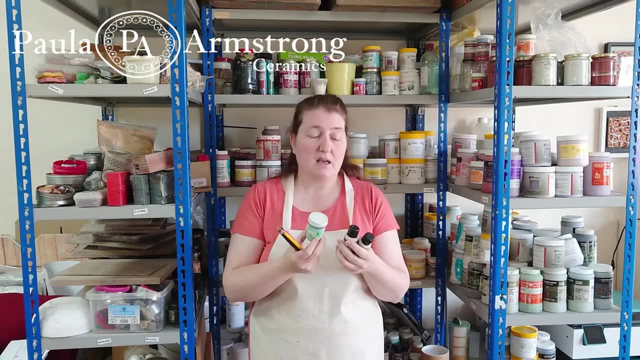 decorative techniques. The other thing about underglazes, particularly the paints, is that you can use them on cream wear or bisque wear. It works at both points, So they're great for adding colour. They generally stay pretty close to the colour that they are. 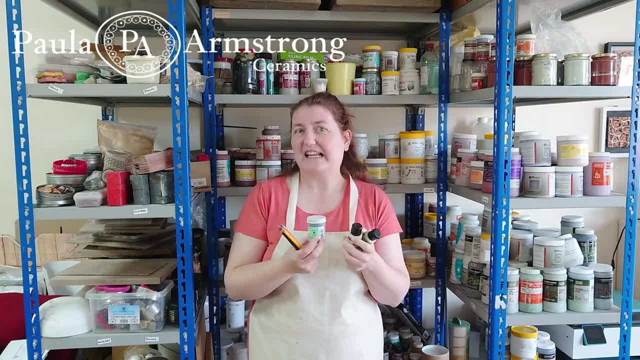 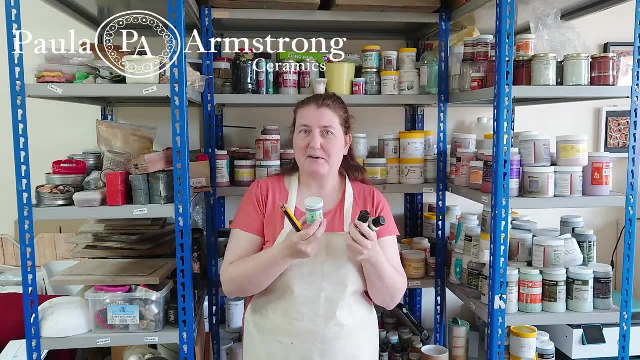 Yeah, they are as well, so they're a little bit more predictable potentially than some of the glazes. so a lot of people like these because they're they're stable, they stay put. you put them on what you draw or what you paint, and that's what. 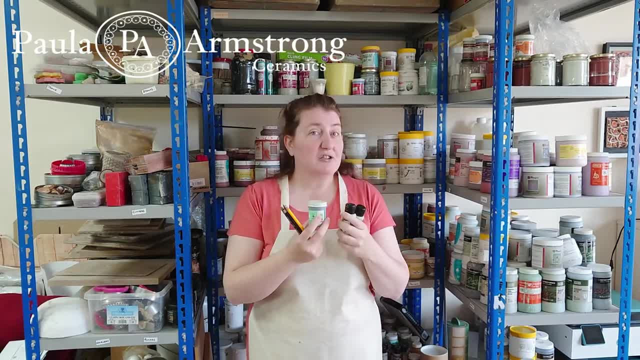 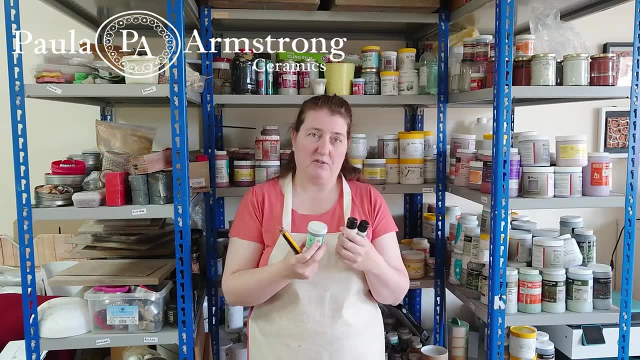 you get at the end of your firing. they are under glazes, though, and they are exactly as they say. you have to put transparent glaze over the top of them to seal them to the surface of the clay if it's going to be on a functional. 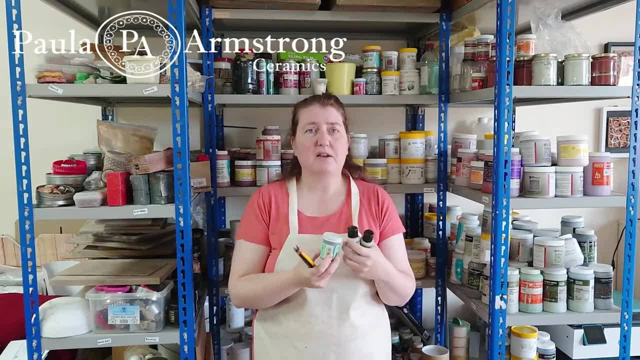 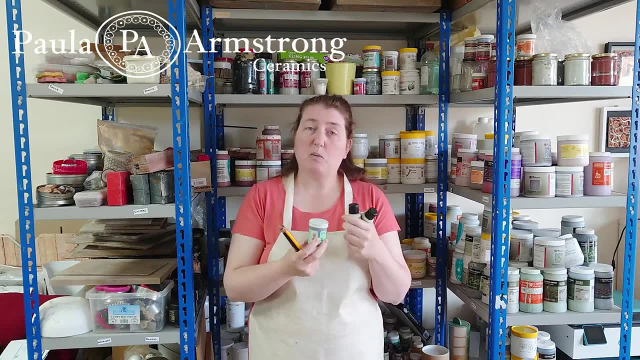 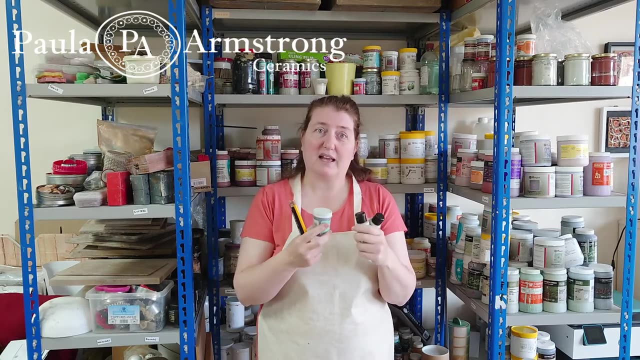 piece. if it's purely decorative, you can probably get away without having a glaze over the top. but be aware that that's a very matte finish. it will mark and it will potentially wear off over time because it's not been sealed to the surface of the clay with the firing, because it is purely pigment, it doesn't. 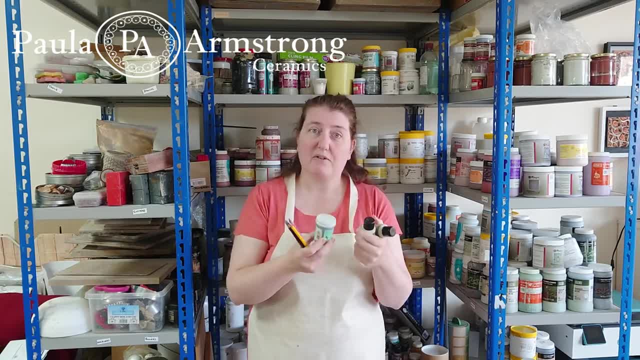 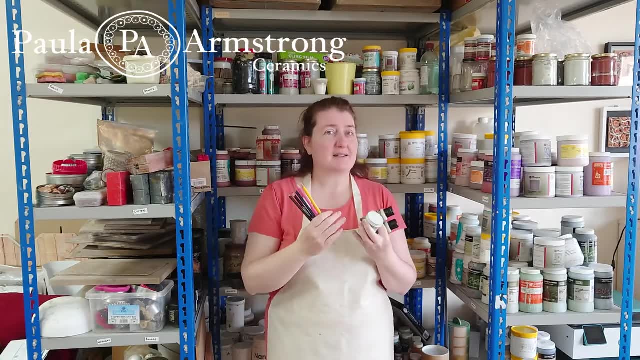 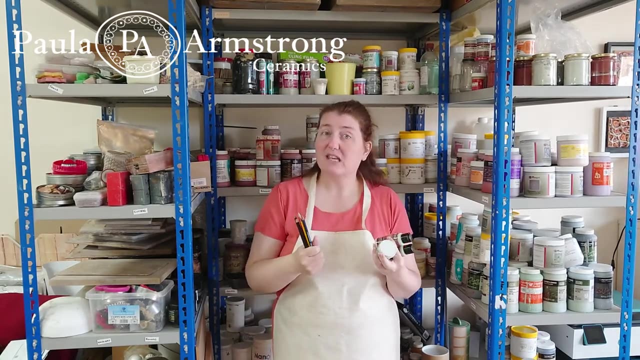 have any silica or any of the other chemicals have. that fixes the colour to the clay. Okay, I hope that helps with all the basics of using under glazes. They're great fun to play with, so go have some fun experiment, try them out, see what you think. Some people prefer them to glazes. 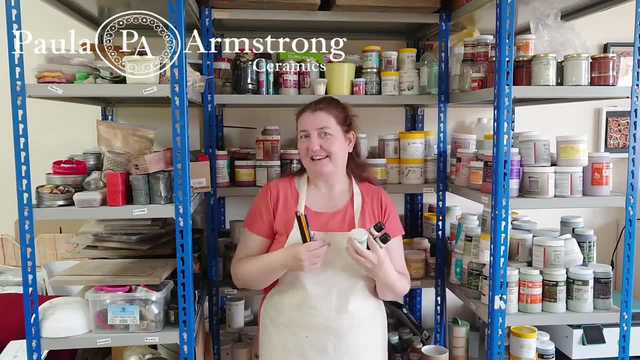 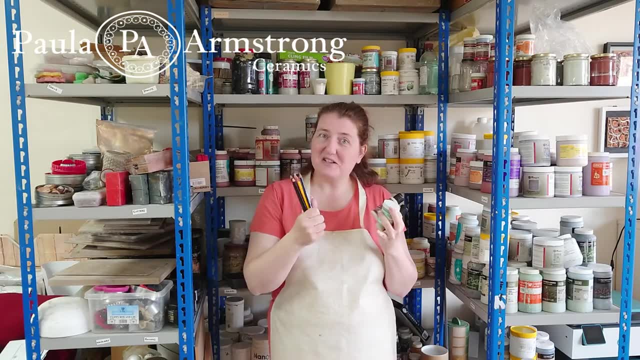 because of the stability and personally I prefer glazes because I prefer the unpredictability and the fact that you can layer up and get some different effects. but the choice is yours. Have fun.